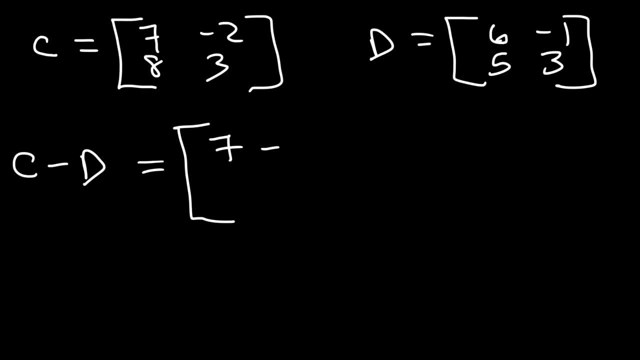 So let's subtract the corresponding elements, It's going to be 7 minus 6, and then negative 2 minus negative 1, and then 8 minus 3, I mean 8 minus 5, rather, and then 3 minus 3.. 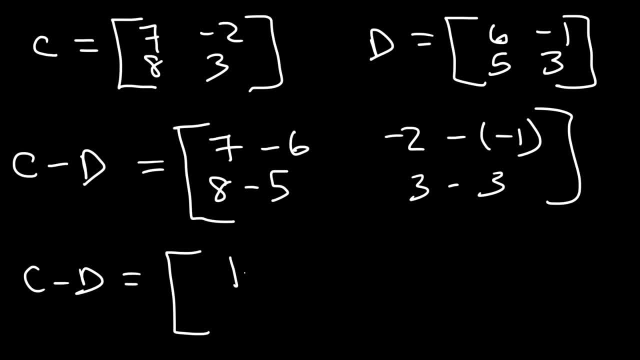 So the difference between the two matrices, 7 minus 6, is 1.. 8 minus 5 is 3.. Negative: 2 minus negative 1, that's the same as negative 2 plus 1, which is negative 1, and 3 minus 3 is 0. 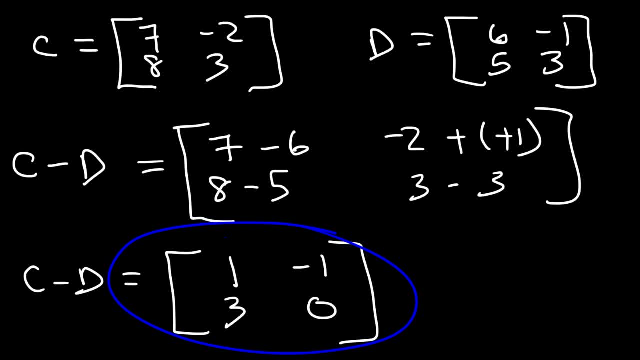 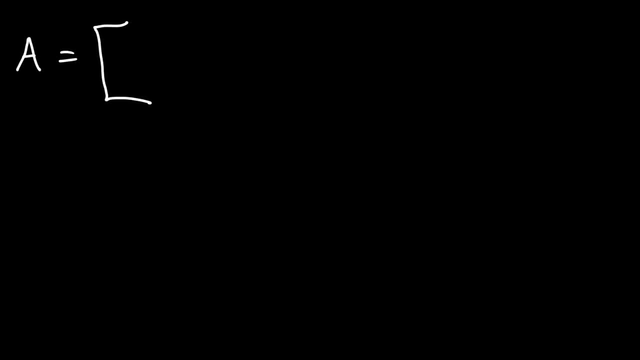 And so that's the difference between matrix C and matrix D. Now let's say, if we have matrix A and we're going to use a 3 by 3 matrix this time, Let me make this a little bigger. So let's say the numbers are 3, 8, negative 5, 4, 6, 2, negative 7.. 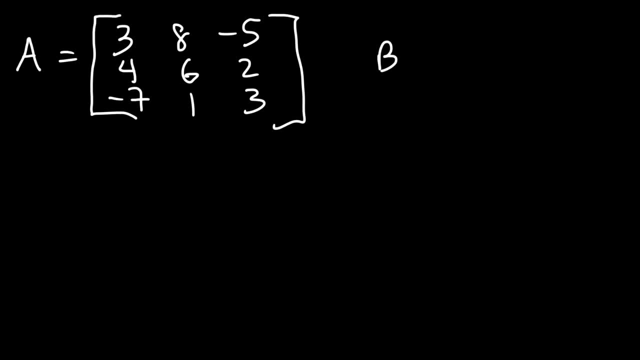 1 and 3.. And matrix B is 4,, 3,, 7, negative, 2,, 8,, 4, and then 3, negative, 5, negative, 9.. Feel free to pause the video. Go ahead and add the two matrices. 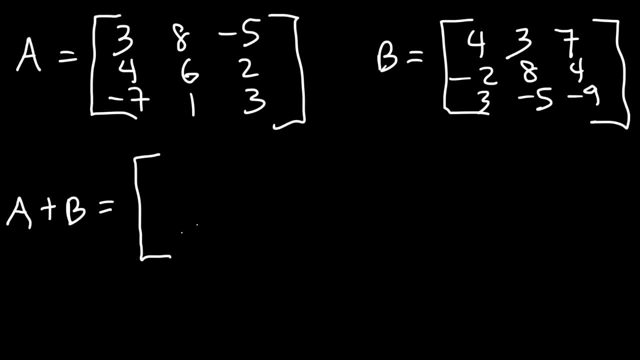 So let's write it out first. So we're going to have 3 plus 4. And then 8 plus 3.. After that, negative 5 plus 7.. In the second row, we're going to have 4 plus 6.. 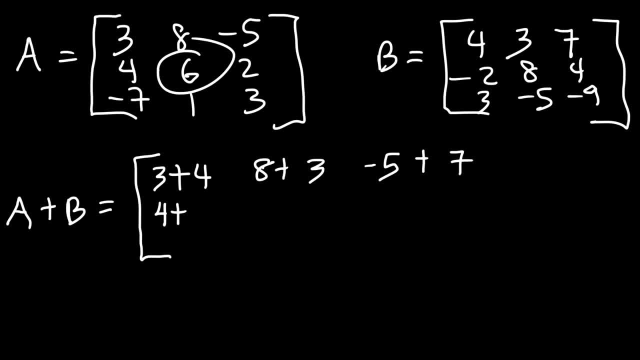 Actually that's 4 plus negative 2.. I was looking at this number for some reason, And then it's 6 plus 8. And then 2 plus 4. And then negative 7 plus 3.. 1 plus negative 5.. 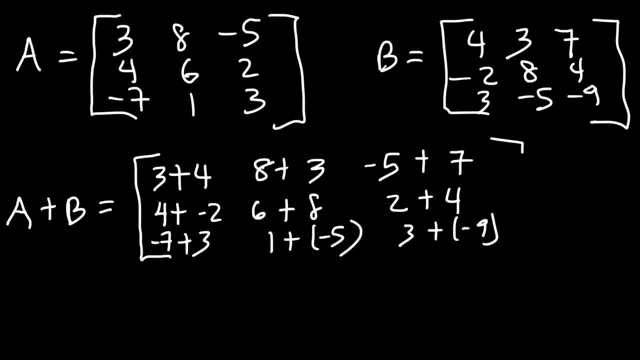 And then 3 plus negative 9.. So let's go ahead and add those numbers. So the first one, 3 plus 4,, that's 7. And then we have 8 plus 3,, which is 11. And then negative 5 plus 7,, which is 2.. 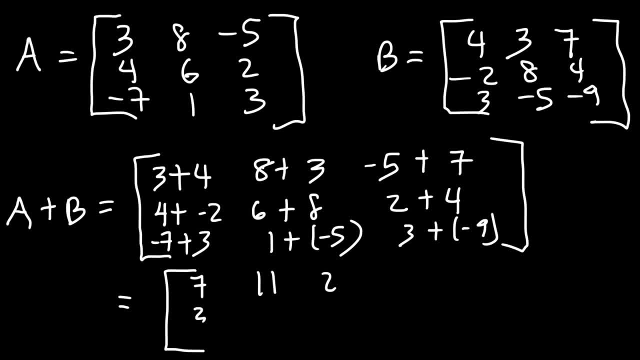 And then it's 4 plus negative 2, which is 2.. And then 6 plus 8, that's 14.. And then 2 plus 4, which is 6.. Negative: 7 plus 3, that's negative 4..